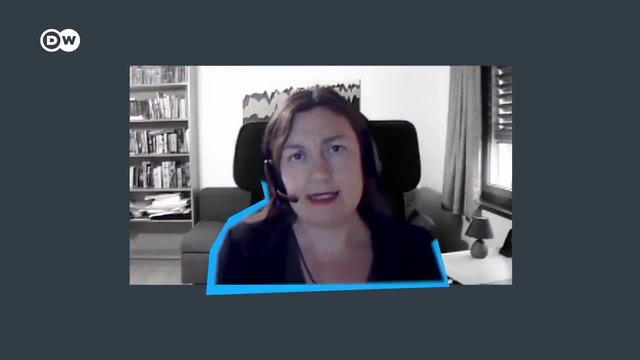 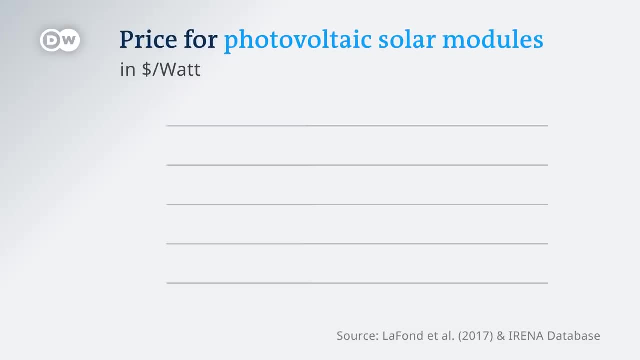 And then I thought solar is ridiculously expensive. Jenny Chase is the head solar analyst at research firm Bloomberg NEF. You'd pay about $4 a watt for a solar panel, And today you'd pay about 20 cents for that same watt. And that is just the last 15 years. 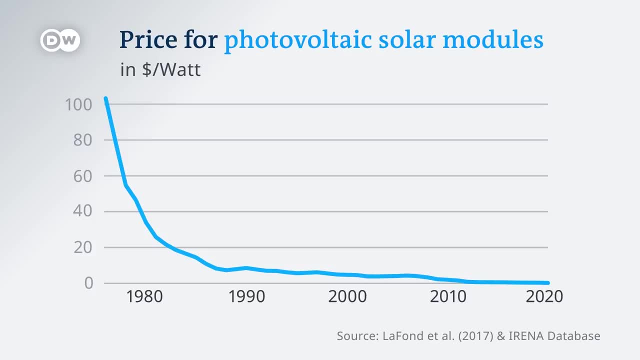 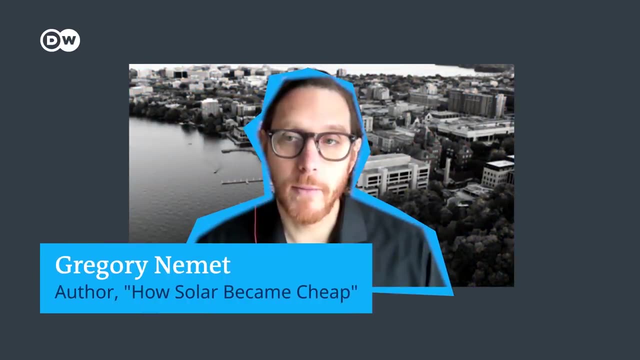 If you think about it, if you look further back, the price drop is even more impressive. How did this happen? It's been a long story, but it's unbelievable. Gregory Nemeth has written a book about this. I know one country did it. 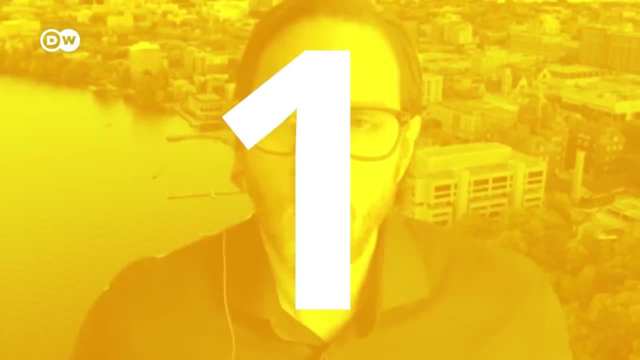 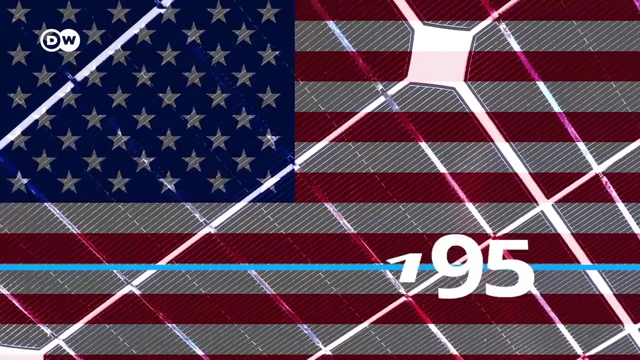 It was an exchange of one country building on another One. the US created the technology. The modern-day solar cell made from silicon was invented in the US in 1954. Back then it mainly got used in the space industry and was still super expensive. 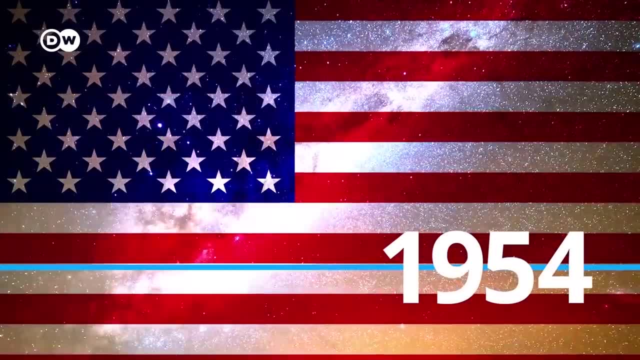 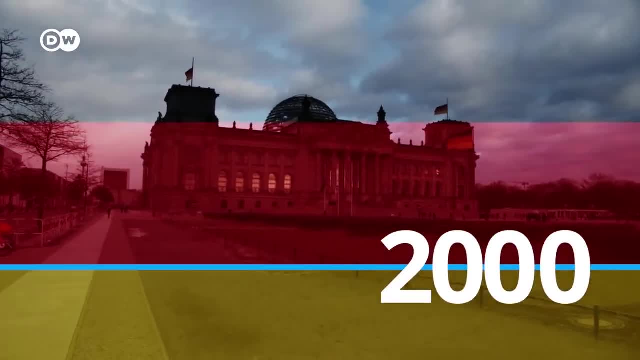 But as the technology progressed, prices started to fall. Two: Germany created a market. In 2000,. Germany passed a law to boost renewable energy development. This was big because it put a fixed price on energy generated from sources like wind or solar. 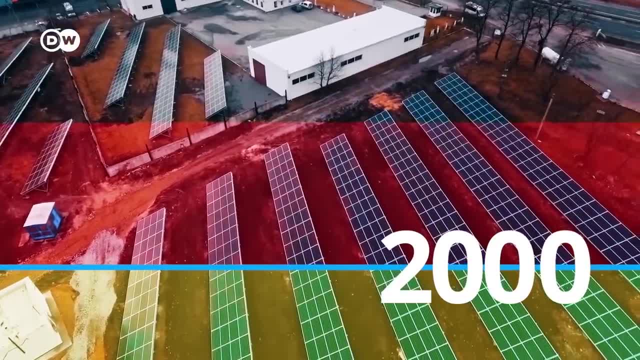 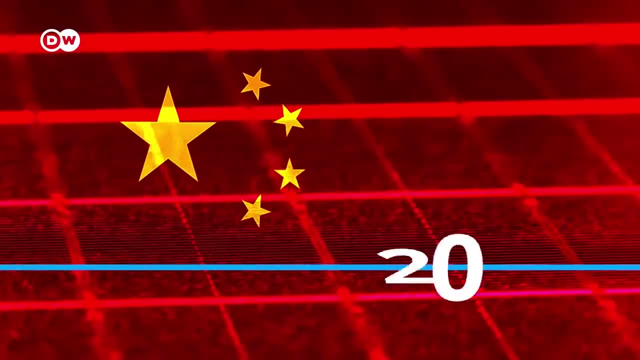 That gave people and companies a reason to set up solar panels. And for them to do that, someone needed to build these solar panels. Three. China made it cheap. Once the German law had come into force, they really started to pump out those solar cells. So basically it built a whole industry for this on a scale that the West really didn't keep up with. China was almost a non-existent player 20 years ago and today they're the biggest producer of solar panels- about 70% of the world's production. 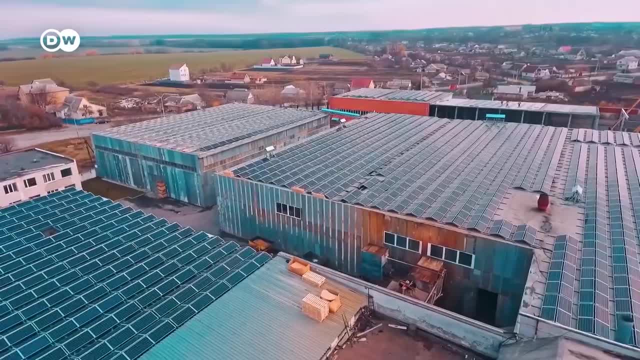 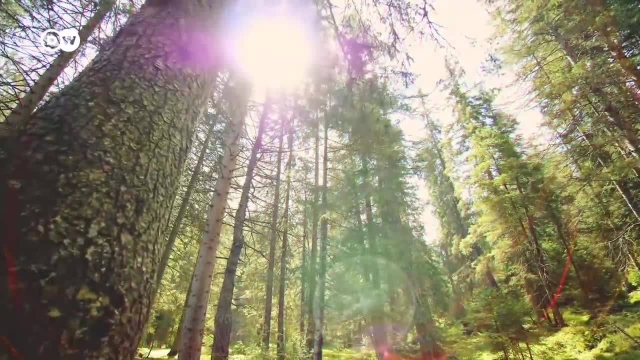 So this is how we ended up where we are now, with clean energy. that also makes business sense. But if solar is so great, why don't we rely on it much, much more and just switch off all these dirty power plants? Well, solar has always had this one big problem. 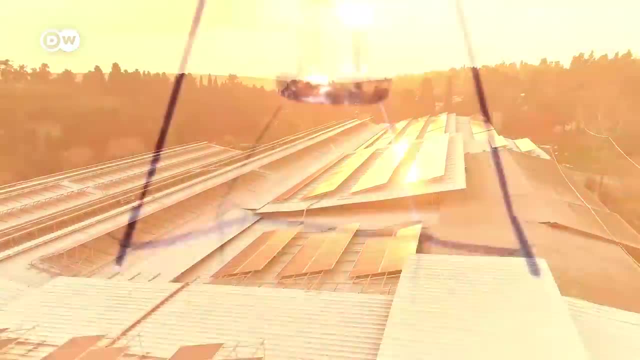 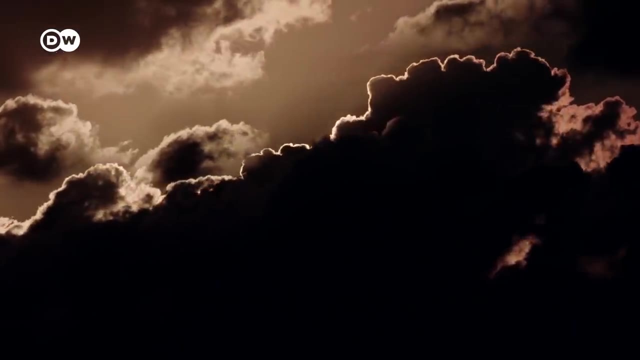 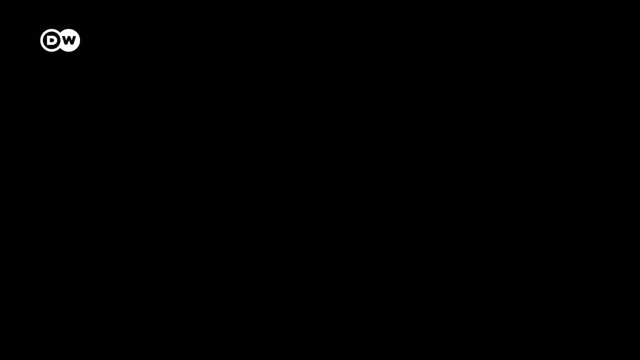 It only really works when the sun is shining. When it's cloudy or, even worse, dark, even the best solar cells are pretty useless, And that's a real shame, because that's when we'd need them the most. Let's take a look at how we use energy. 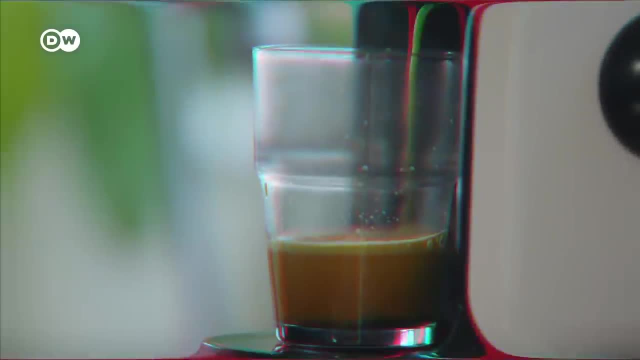 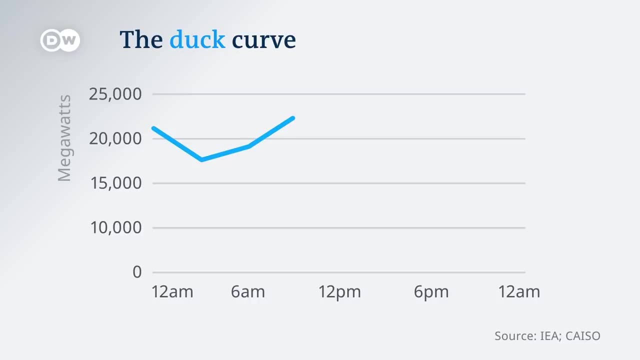 In the morning, when most people get up and get ready, we need energy. The so-called duck curve charts our demand for power from non-renewable sources like coal and gas throughout the day, first in places without much solar. After the morning spike it stays pretty level. 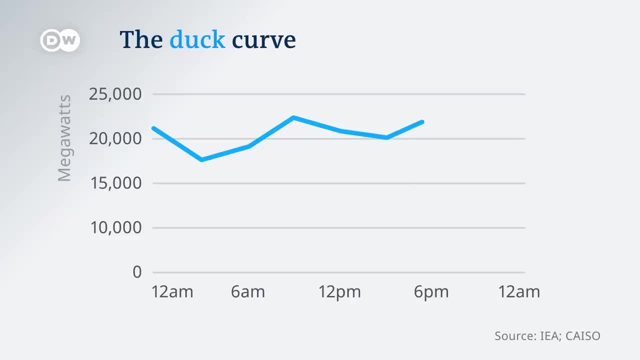 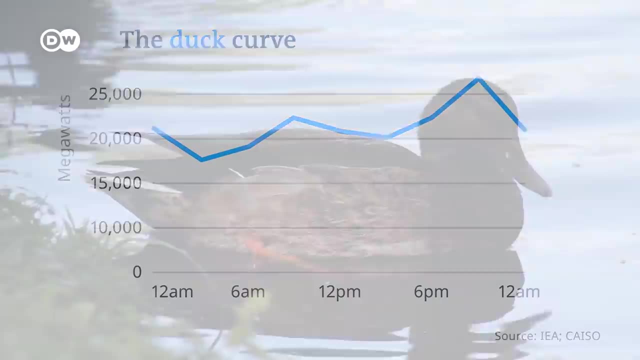 When people come home in the evening it goes up again and then drops at night. At this point you might get an idea why they call it the duck curve, because it kind of looks like a duck. Anyway, in places with lots of solar, 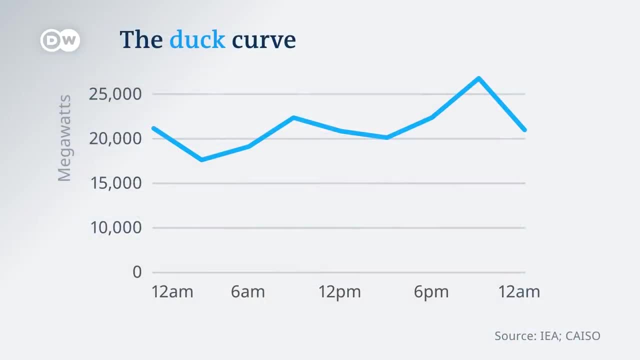 like California, this curve changes. The mornings are pretty much the same. Then the sun rises and solar energy production kicks in. This lets demand for non-renewable energy drop Until the sun sets, that is. That is when conventional demand shoots up again. 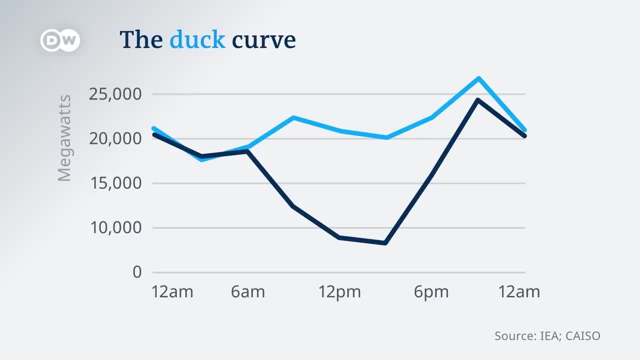 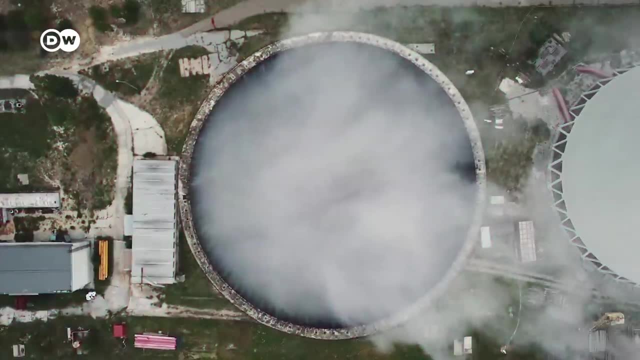 way steeper than in the first curve. Two problems with this: One: traditional power plants suck at ramping up this quickly. That means you have to keep them running at a certain output all day, even though there's lots of solar. That means You can end up with actually more power produced in the middle of the day than is used, And that leads to the second problem. There are limits to how much energy you can put into the grid. Too much solar could overpower it, so it needs to be thrown away. 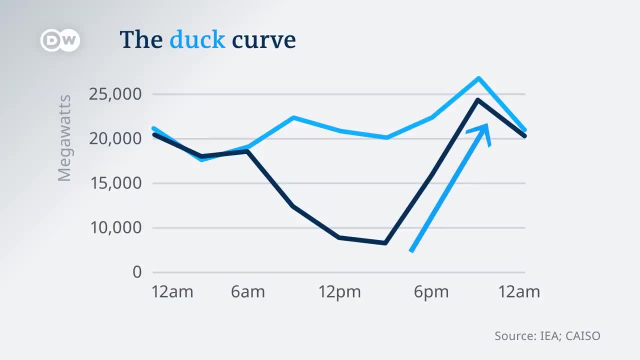 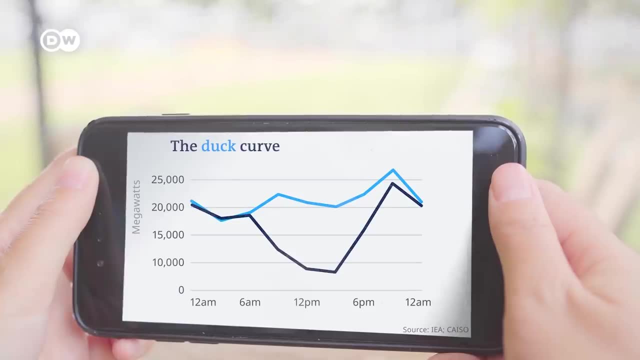 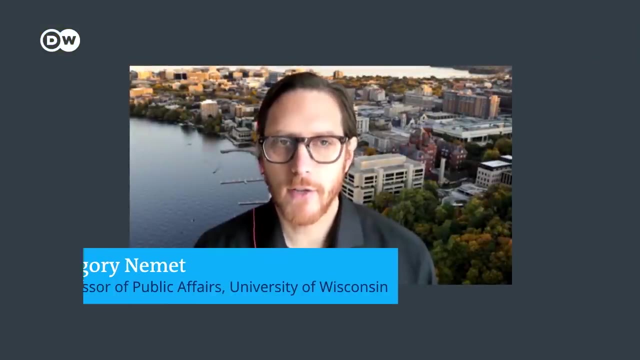 This has always made it super difficult to add lots of solar to power systems. But guess what? There is now a solution to this And chances are you have part of it in front of you right now: A lithium-ion battery. We're just taking that same construction. 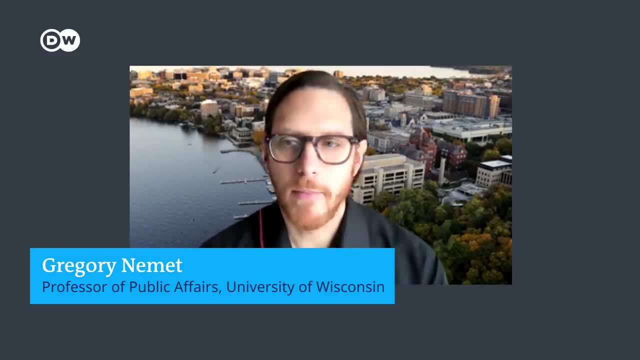 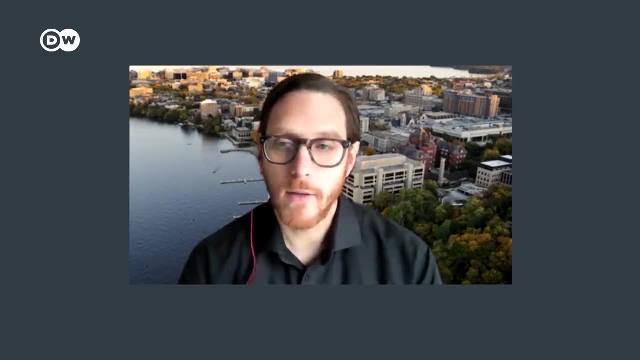 stringing together many, many of those cells and making battery packs that we can use for cars, And then we can also scale that up to use for stationary power to go next to wind parks or solar farms. What's been quite good over the last few years. is that batteries have got a lot cheaper as well, And we're now seeing solar projects built with a couple of hours of storage in the battery, so that they can shift Solar generation from the middle of the day to the evening, where there's often a peak in electricity demand. 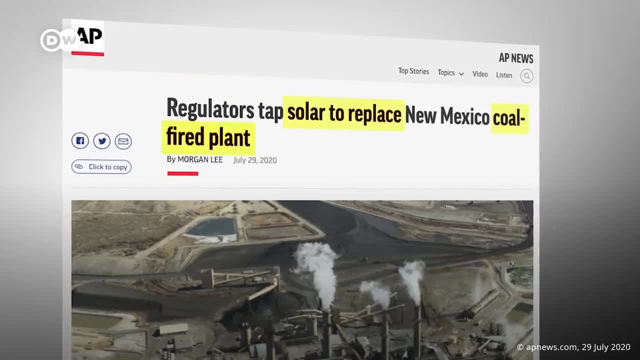 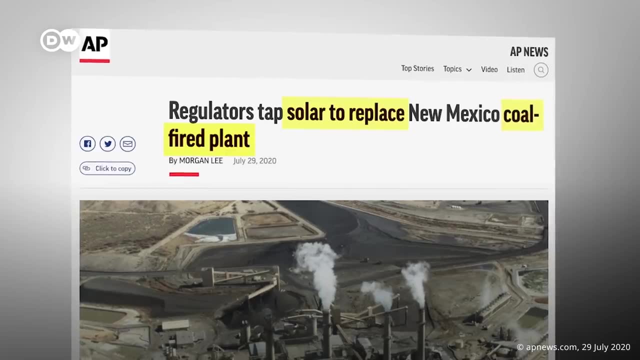 In the US, for example, the state of New Mexico just decided to shut down a coal plant and instead build new solar farms that store large amounts of the energy they produce in batteries. Lithium-ion batteries have become a lot better and a lot cheaper than expected in the last few years. 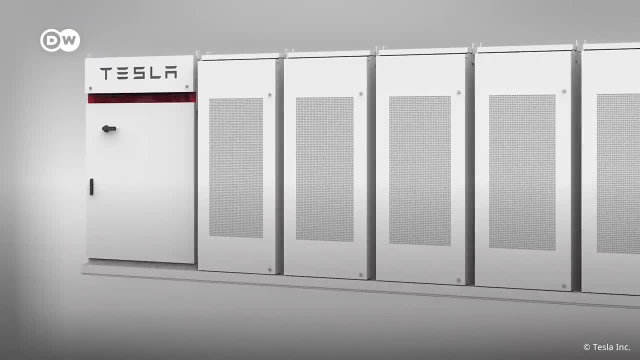 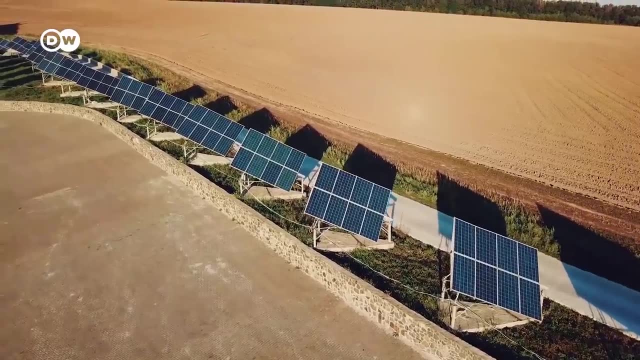 They're now a viable option for storing and shifting at least a few hours' worth of solar energy as needed, So the storage problem that solar always had is actually not that much of a problem anymore. Sometimes, though, we might want longer-term storage. 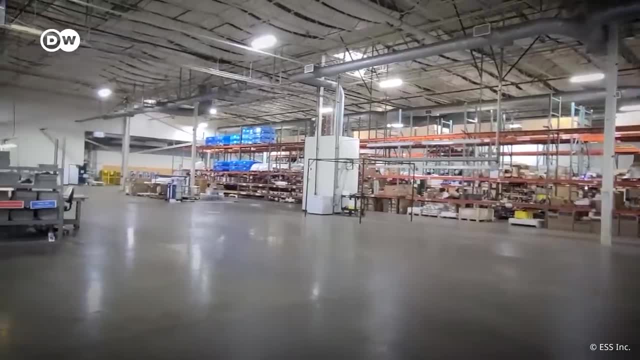 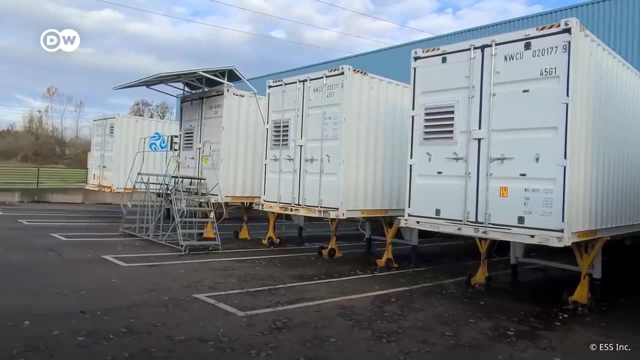 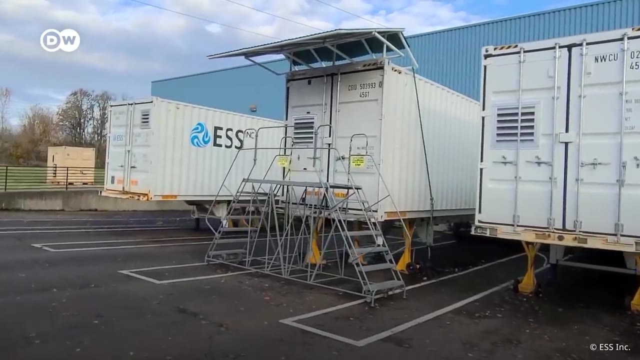 in places without much sunshine, for example, And that's why companies are offering other solutions. Let's just run through a few. Another type of battery, called a flow battery, separates the charge outside a cell. That has two advantages: It can store more energy, and for longer.